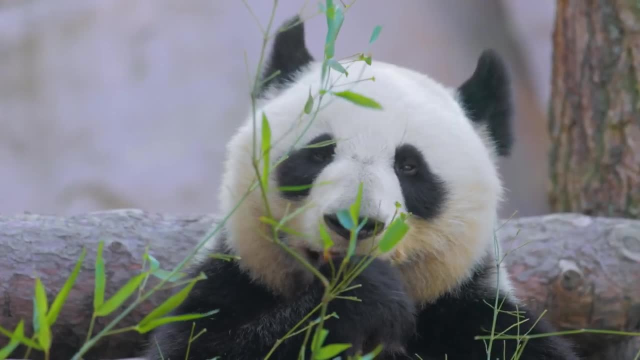 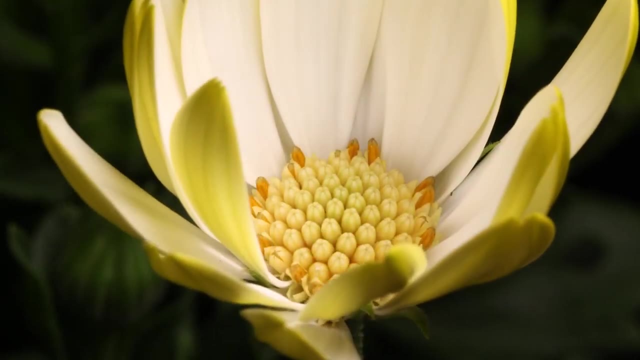 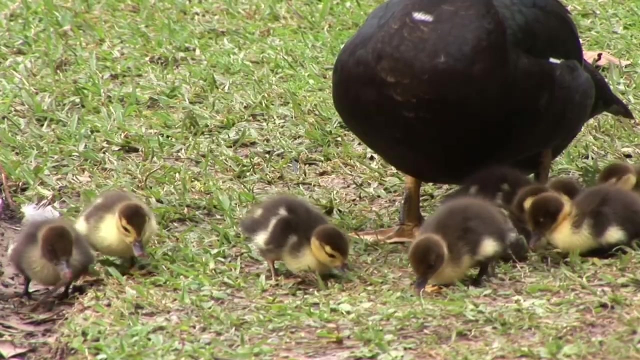 give the plants and animals a chance to explore the world. Plants and animals live in places that need to survive. Plants get the sunlight, water and air they need to grow. Animals find their food, water and air in the places they live too. Now think about your favorite animal Where. 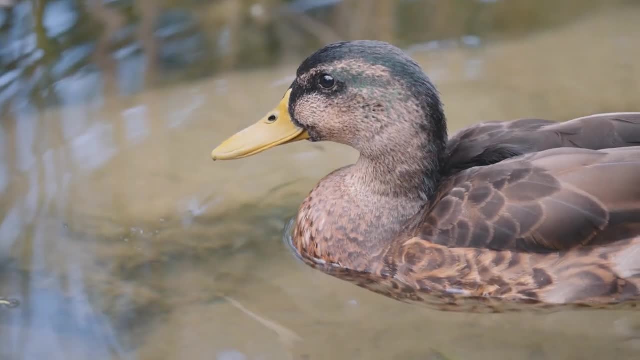 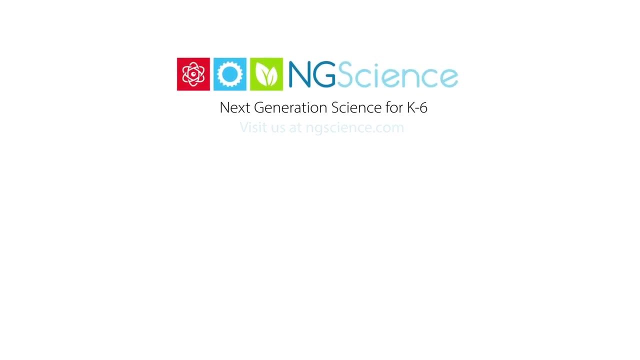 does it live And how does it get the things it needs to live and grow? Don't forget to subscribe. 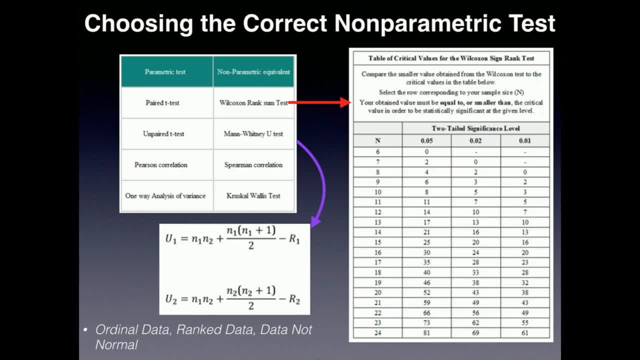 Welcome back to Statistics on Catalyst University. My name is Kevin Tokoff. Make sure to like this video and subscribe to the channel for future videos and notifications. So in the first, probably half of this playlist, the kind of statistical tests that we've been using are what are referred? 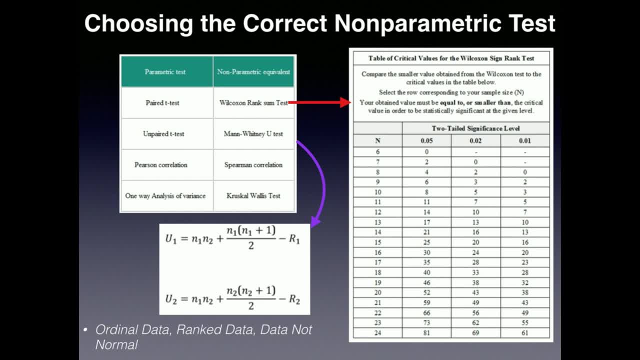 to as parametric tests. They tend to be the most common tests that are covered in most science courses, whether it's biology, chemistry, etc. And those tests are parametric, which means there's a lot more stringent and rigorous assumptions that go into the actual population. 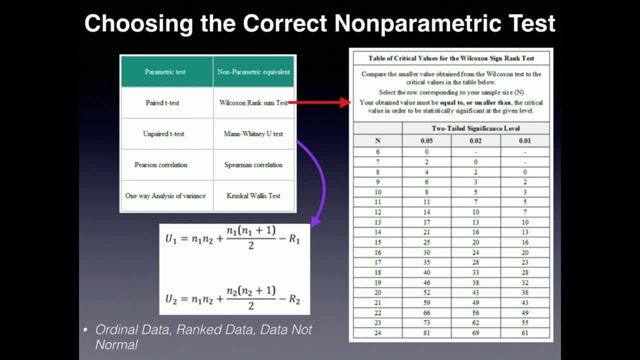 and the data and so forth, And one of those important stipulations is that the data is normal. Now, what do you do if the data is not normal, if it's not a normal distribution? Well, that's one of the criteria that would cause you to use a non-parametric test, And 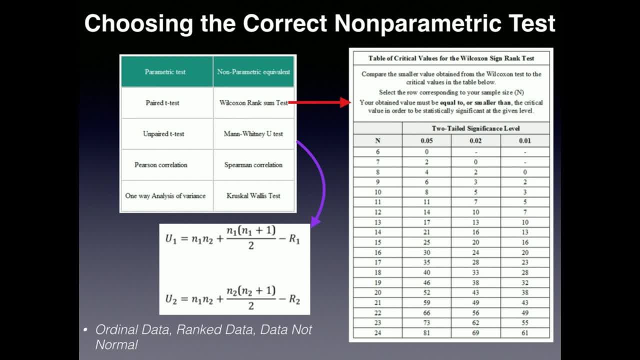 we're going to start going over some of these, These non-parametric tests. Now I'm going to say this: These: generally, unless you have some special program like SPSS or something like that, these have to be calculated by hand. In the Excel add-ins you do not have these options for doing non-parametric tests.